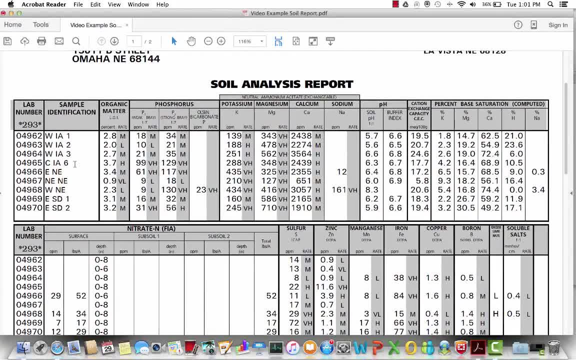 at some soil test results and I've got about 10 soil test results, nine soil test results and I'm coming from some soil samples in western Iowa, central Iowa, eastern Nebraska, northeast Nebraska, western Nebraska and a couple here in eastern South Dakota. So we've got a kind of a. 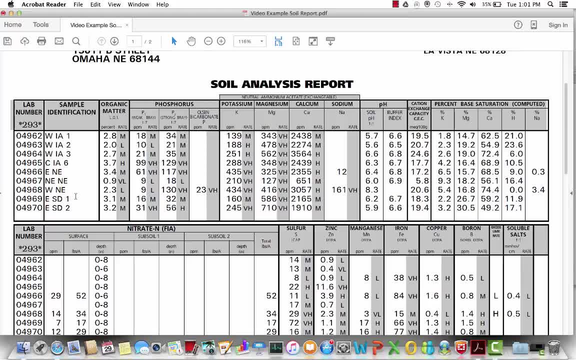 wide variety of soils With different textures, different pH values, different fertility levels. So we can kind of look at a wide range of different samples and you might say, well, you know these, these sample areas aren't real close to where I farm. Maybe I farm in Indiana or Illinois or Montana, Colorado. 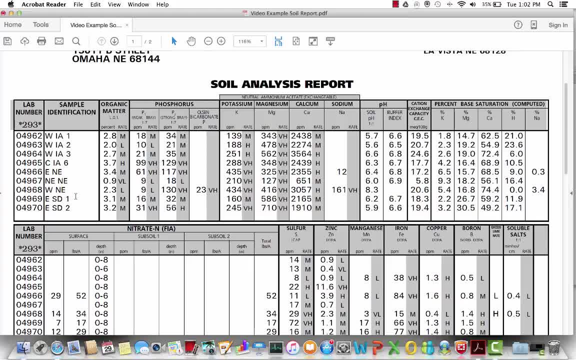 I would say that you know, stick with me here and we'll walk you through some of these, and I think you'll find a lot of these ideas would also apply to soil samples from your farm. The numbers may be a little bit different, but the the way to go about interpreting the results, I think. 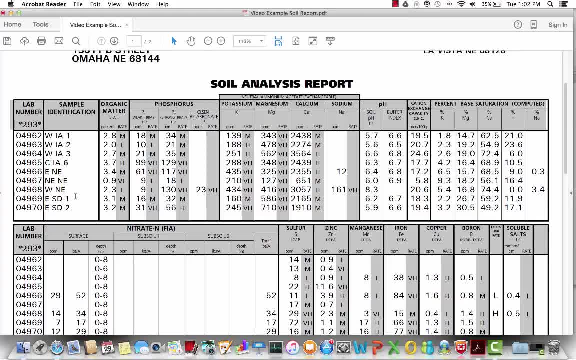 is going to be very similar. So when I start looking at soil samples for the first time, especially if I'm not real familiar with the fields that I'm looking at or the area that I'm looking at, I always start at cation exchange capacity. We see that over here a little bit. 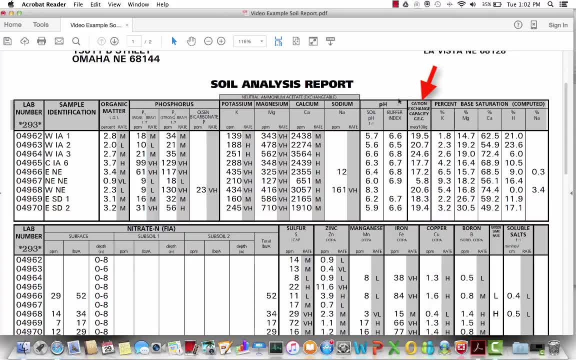 to the right side of the report in the top section Cation exchange capacity or CEC. Cation exchange capacity is a measurement of the exchange sites on the soil, So it would be the negatively charged exchange sites that are holding cations. We get that number at the laboratory by 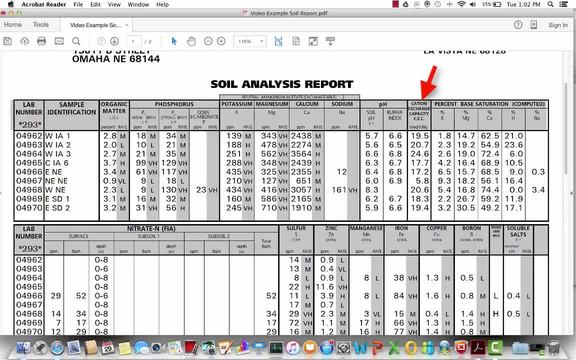 doing this neutral ammonium acetate extraction to bring out the cations, and then we measure those on an instrument and then there's an adjustment made for the molecular weight and the charge or valence of those cations And then we also look at the amount of hydrogen that's coming off of our pH and our hydrogen. 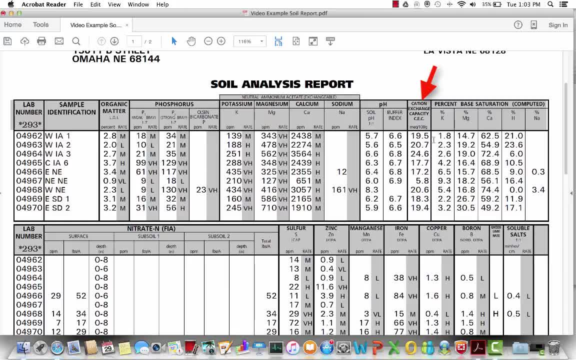 percentages over here. That all goes together to calculate a cation exchange capacity. Generally speaking, the lower the CEC, the less nutrients and water the soil will hold, And the higher the CEC, the more nutrients and the more water a soil will hold, And it's very. 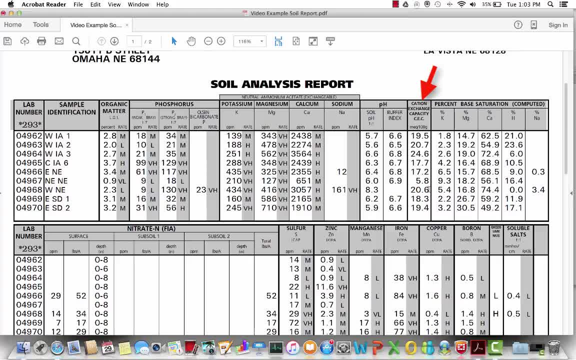 related to the texture of the soil. The higher the CEC the more clay is in that soil. The lower the CEC, the less clay and oftentimes the more sand in that soil. So as you think of soil texture and sand, silt and clay, you can kind of think of very low CECs like this. 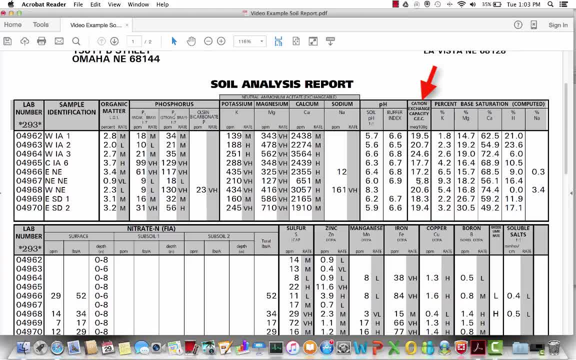 five we see in this sample from northeast Nebraska. It has a very low CEC, probably has a fairly high sand content in that soil- Our highest one on this report from western Iowa- with a cation exchange capacity of nearly 20%- The lower CEC. the lower CEC has more clay in it and is probably a silty clay loam type soil and will. 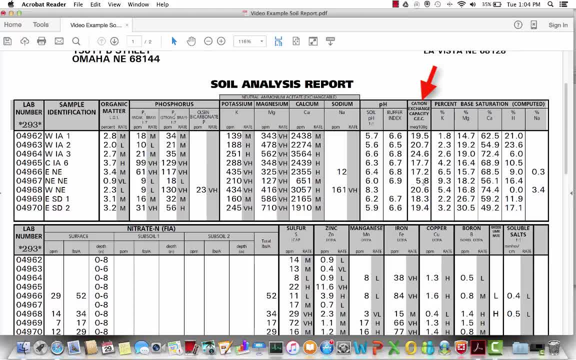 hold quite a bit more water and nutrients than the sandy soil we see here from northeast Nebraska. As you think about CEC, you kind of want to understand the differences as you go across a field to see if there are areas that maybe should be managed differently. As I look at these lighter 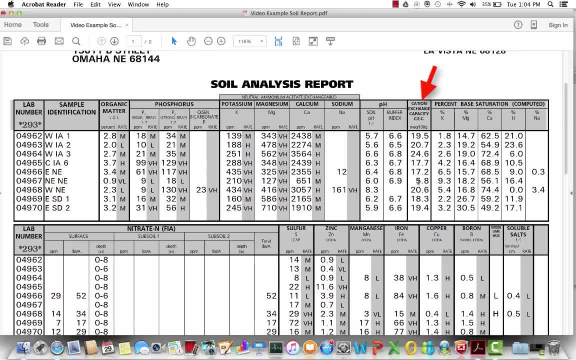 soils, which refers to a sandier soil with a lower CEC. I know that it's going to hold less water. If I were managing irrigation on a field that had this range of cation exchange capacities, I'd know this area, with the CEC of around six, is going to hold less water. the plants in this area. 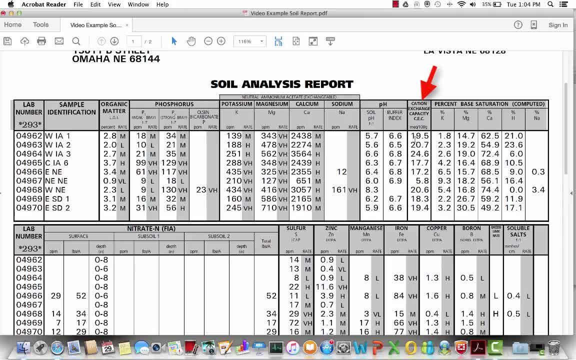 are going to wilt faster, And, as I look at managing the irrigation for the field as a whole, I'd probably want to not just turn on the pivot when I see these plants in this area start wilting, because So I'm probably going to apply too much water in this area and we're going to have issues. 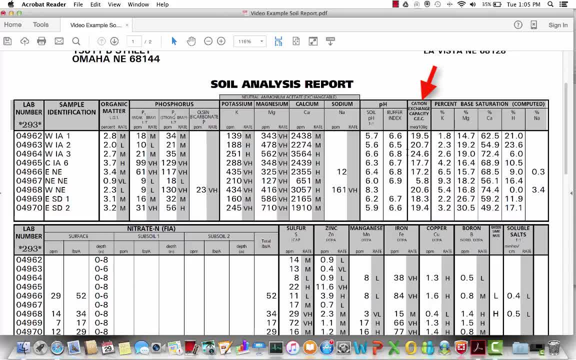 with the field drowning out or a lack of oxygen to the roots of the crop in this area. So we think about water holding capacity in CEC a lot. We also, of course, think about nutrient holding capacity and also the ability of the soil to supply nutrients beyond what we'll see in the rest of the analysis we look at. 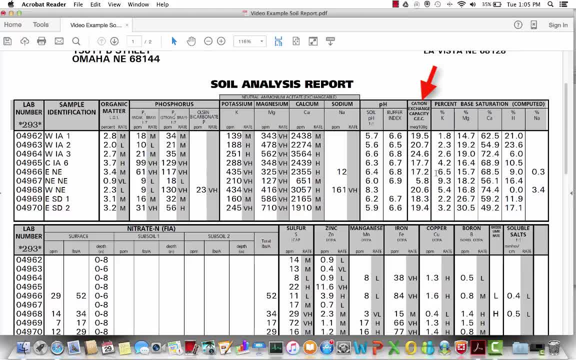 But a heavier soil generally is going to hold more nutrients and supply more nutrients than a lighter soil. It's also going to have more likelihood of nutrients that we do apply being tied up in the soil and a little less available to the crop. So as you look at this CEC of nearly 25, there's probably more nutrients in this soil but they're. 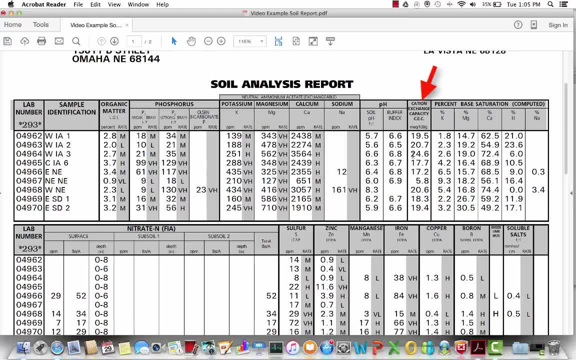 also more likely to be tied up. Now, of course, we're going to look at phosphorus, potassium, sulfur, the micronutrients, to see what those nutrient levels are, But as we think about how the nutrients that we do apply in addition to what the soil can, 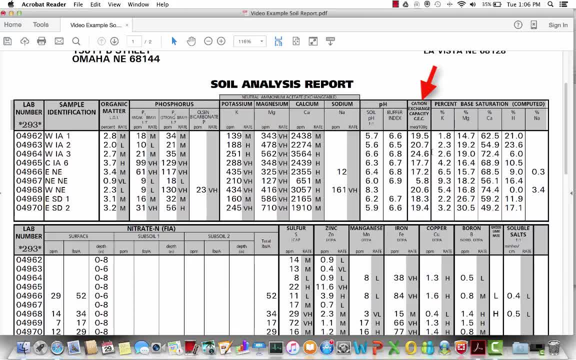 supply are going to be handled. We need to think a little bit about that CEC and how tie up versus available nutrients might be affected by that soil texture. After looking at CEC for a little bit and getting a good feel for where I'm at and generally, 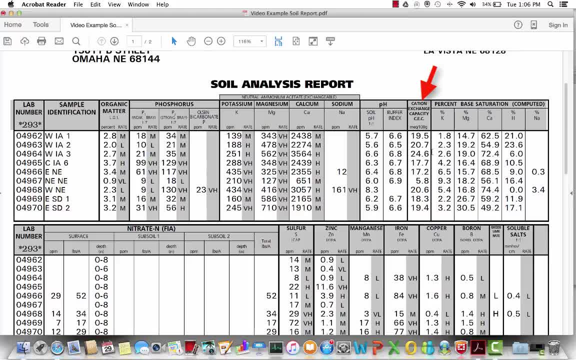 in the area that I work a lot of- Iowa and Nebraska- we get a lot of CECs between 15 and 25. But I also see outliers. quite often I'll be dealing with a field that might have a CEC range, mainly between 12 and 17.. 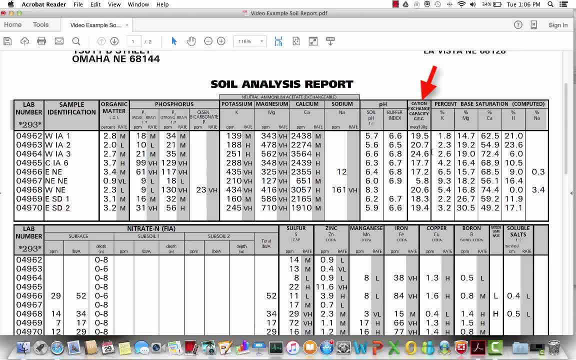 So that's a good feeling. for where I'm at and generally in the area that I work- a lot of Iowa and Nebraska- we get a lot of CECs between 15 and 25. But I'll have an outlier with a CEC of 25, well, it's an area that, for whatever reason, 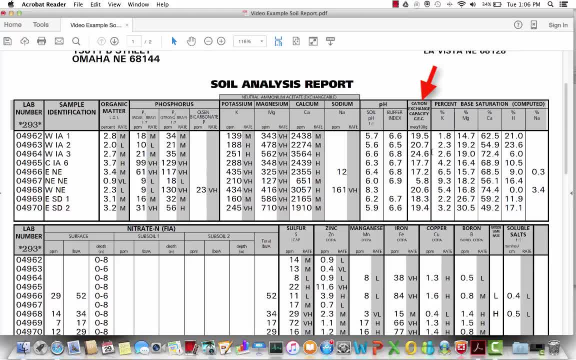 has a lot of clay in it, Or maybe I'll be dealing with a soil that has a CEC range of 15 to 22,, but I'll have an outlier that's sitting around 4 or 5.. And what a lot of times it will tell me, I should do is maybe pull up an NRCS map and 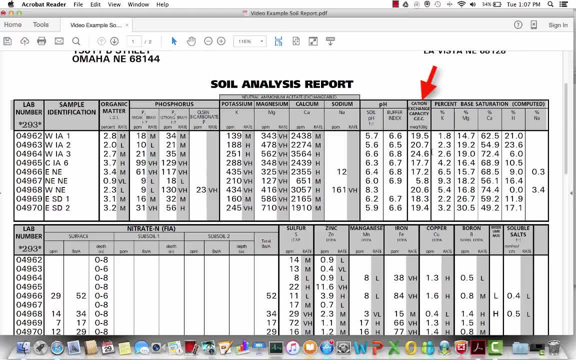 see if I can understand from the soil survey what this difference is, that I'm looking at and understand how big that area might be. it's really an indicator of what additional management things that you would want to do on a field like this, based off where you see the variation in. 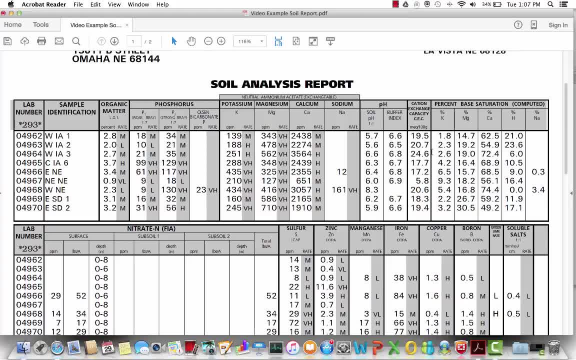 cation exchange capacity. So after CEC, I generally move over to organic matter, and again we're still in that same line of thought: What is this soil's ability to supply nutrients, and how much am I going to have to supplement the soil's natural ability to hold and supply nutrients with applied fertilizers? So 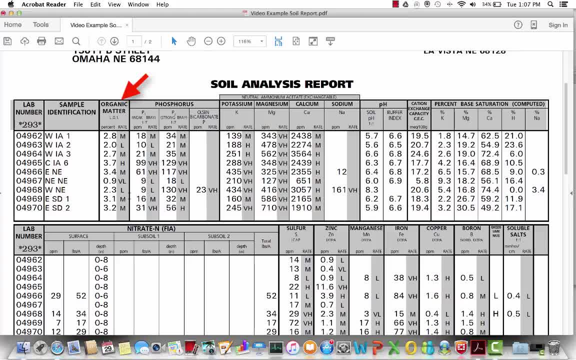 from organic matter. of course we know it'll supply some nitrogen, it'll supply some sulfur. a lot of micronutrients can be supplied by the breakdown or mineralization of organic matter. So I'm looking at kind of a level and is there a big variation in the level in these soils? How much organic matter do I have? 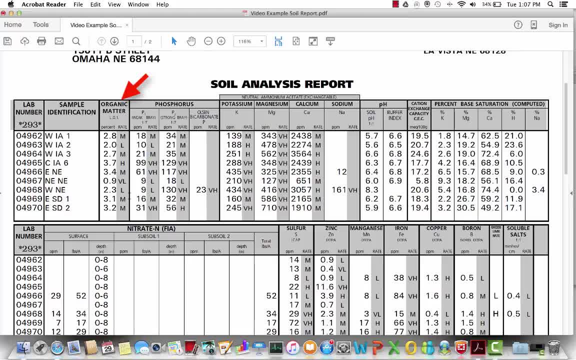 there. Do I expect that organic matter to mineralize through my growing season? If I'm dealing with a cool season crop like wheat, there's probably gonna be less mineralization. it becomes a little less of a factor In a warm season crop like, say, corn or soybeans- alfalfa, I would. 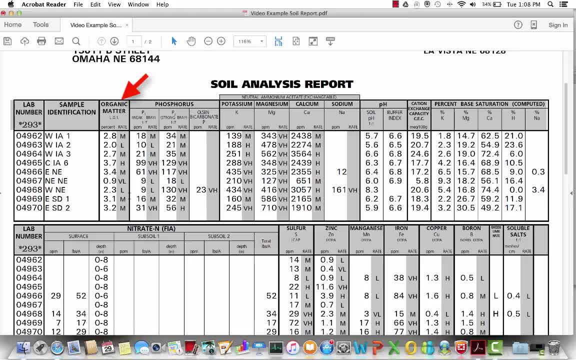 expect, you know, through the growing season, some of those nutrients to mineralize. For an example, from a nitrogen standpoint at the laboratory we're going to credit our normal nitrogen recommendation about 10 pounds for every percent organic matter we find over here on the soil. 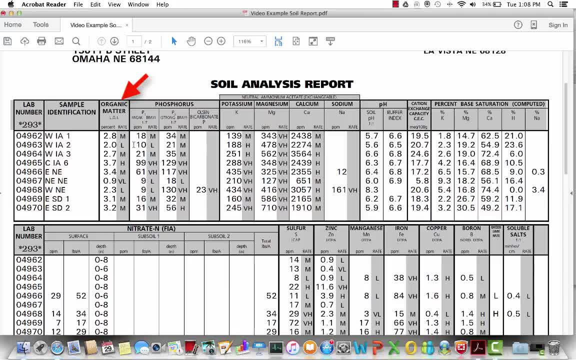 test. Now that doesn't mean that that's the total amount of nitrogen we would expect to mineralize from that organic matter. It's just what we're going to take off of our base rate based on the amount of organic matter we find in that soil. 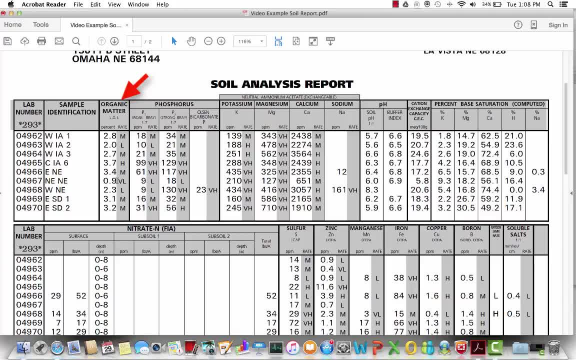 So an organic matter percentage of 0.9 is going to release quite a bit less nitrogen than an organic matter of 3.7, and our adjustment would only be about 10 pounds here in the 0.9, where it would be close to 40 pounds here. 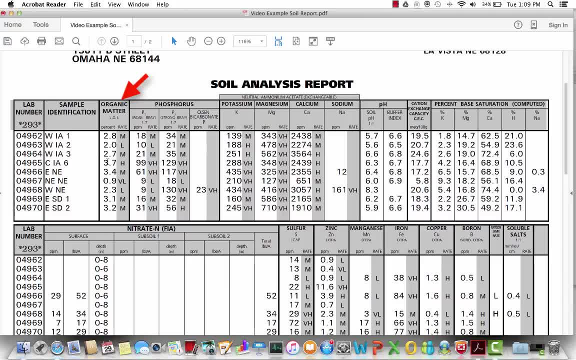 with that 3.7% organic matter. Some of the things I might think about with organic matter would be the workability of the soil or the soil's structure, beyond just its texture. So is it water going to infiltrate? well, A lot of times it can be related to organic matter. 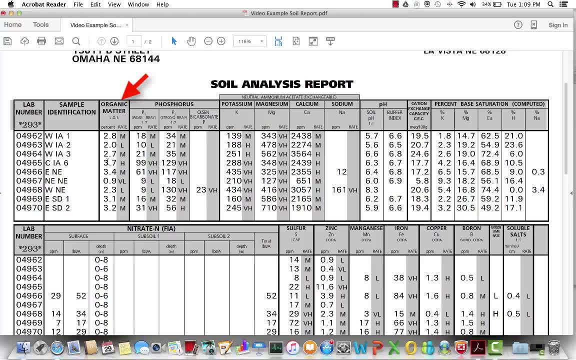 Some of the soil health and the biology of the soil can be related to organic matter. The flip side of that is sometimes we'll see very high organic matters in soils that really aren't all that healthy. Maybe there's very poor aeration. 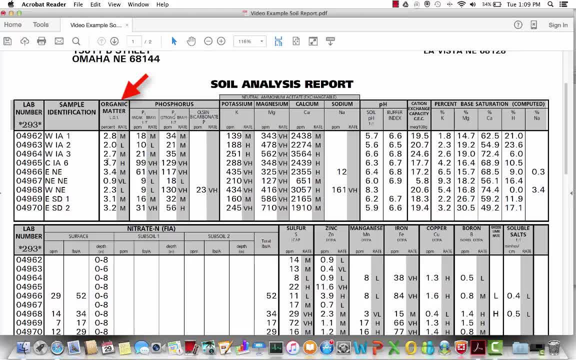 so the organic matter does not break down very readily at all and instead over time builds with crop residues that are added and you'll get some higher organic matters. but the soil's very wet plants don't grow well there, so it has some additional challenges. 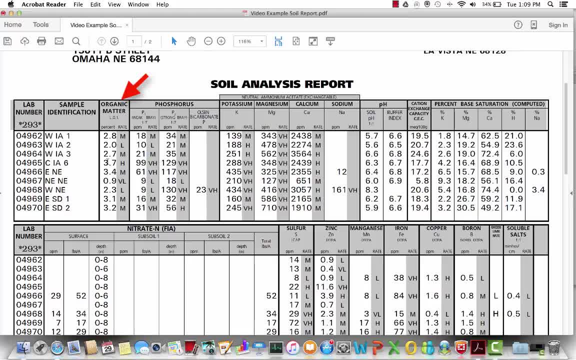 The numbers coming back from the soil test analysis just give you some clues about things that you might want to think about with that soil. As we look across these soils here on the CEC side, we see some concerns. we see some inconsistency between that 15 and 25,. 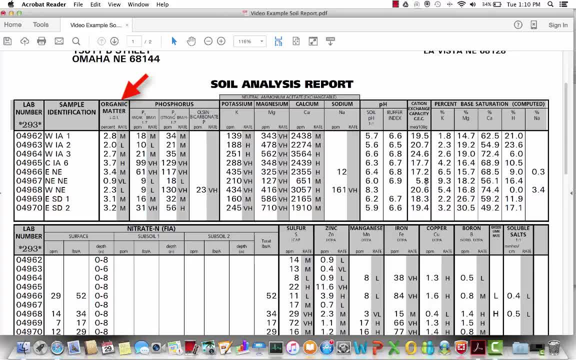 you know, our outliers are the 25, and an outlier here, of course, at only 6.. So between 15 and 20 is going to catch a lot of these soils. but I've got a couple of areas that are certainly outliers. 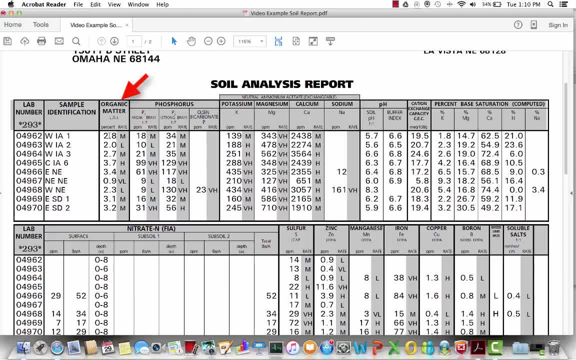 if this were all in the same field, which of course it's not. And then on the organic matter, you know you've got areas that are going to have a lot more ability to supply nutrients with these organic matters in the 3% range. 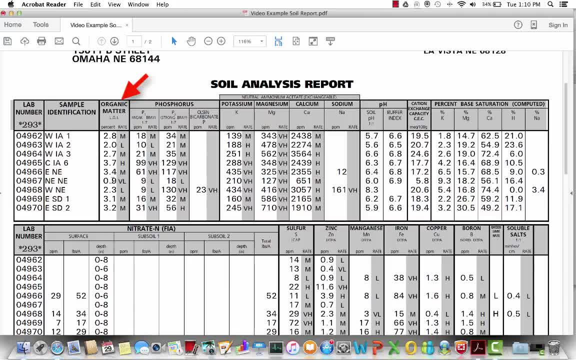 but you've got this outlier that's at less than 1% and you certainly would have to think more. but you've got a couple of areas that are going to have less than 1% and you certainly would have to think more about spoon-feeding nutrients to that soil. 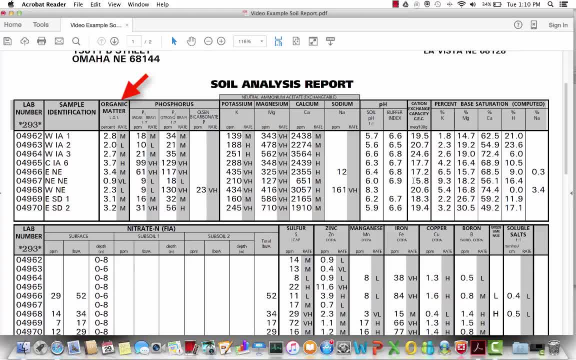 especially when you see that it's also a very light soil as far as CEC is concerned and probably has a high percentage of sand. It's probably not going to hold nutrients very well, nor is it going to have much being supplied from its organic matter. We actually see this quite often- that a very low CEC soil with a lot of sand in it will also have a very low organic matter. The sands have very large pores between those sand particles. It allows a lot of oxygen into the soil. 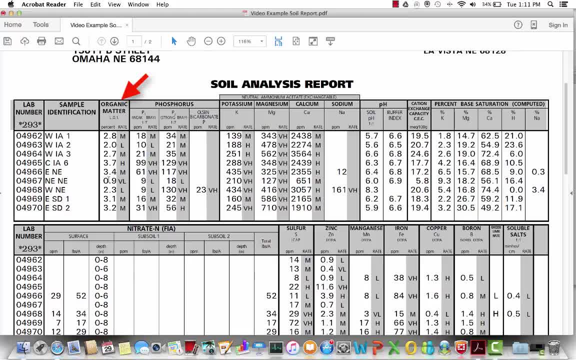 and it makes it so that a lot of times it kind of burns off its organic matter and won't build organic matter very easily and has burned off a lot of what organic matter or organic stover has been added over the years. So after looking at cation exchange capacity and organic matter, 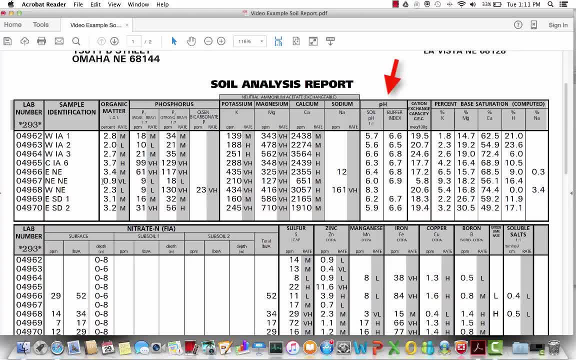 I'll generally go look at soil pH. I've got two pH numbers over here and they create a lot of confusion: The soil pH, the 1 to 1, and as you see across the top here, you can see the. 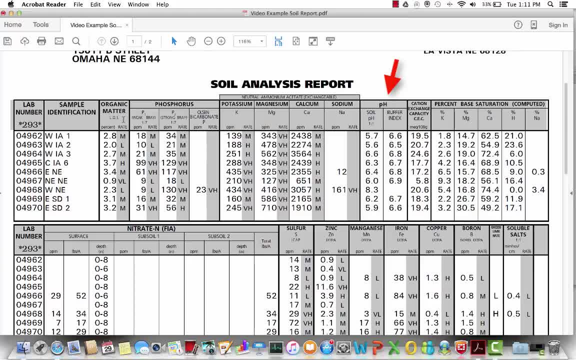 analysis that we're running or the methods that we're using to do our analysis. It'll say across the top: like LOI is loss on ignition for organic matter. We see the P1 weak bray, the P2 strong bray. 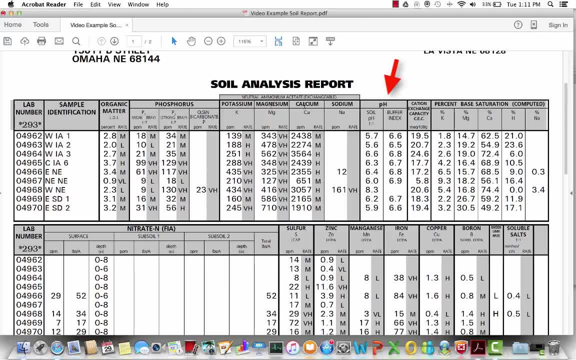 the Olsen bicarbonate test For all the cations. we're using this neutral ammonium acetate extraction On the soil pH. we're using a 1 to 1 ratio of your soil with distilled deionized water And then we put in a 1 to 1 ratio of your soil. 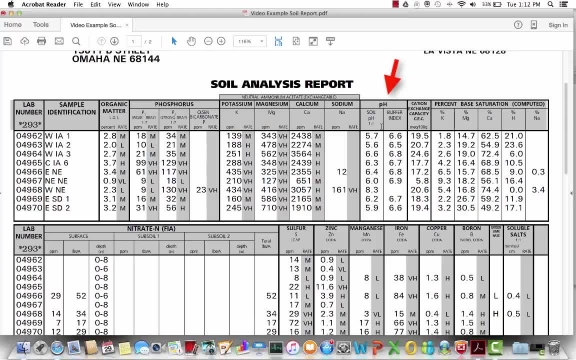 and then we put a pH probe in there and we measure that pH directly. So of course you need to know what pH works best for the crops that you're working with, But a lot of times for, say, corn and soybeans. 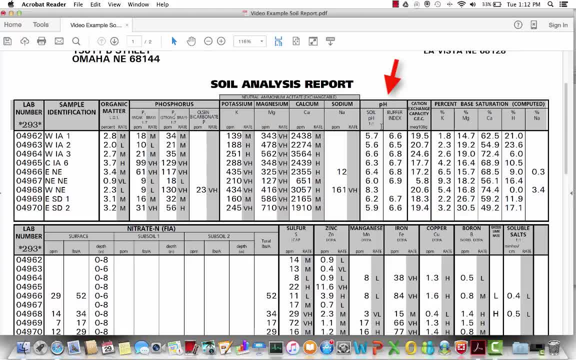 something in that. 6.5 to 7.2 is a really good range. If you're dealing with something like alfalfa- sometimes a little bit higher, maybe- a 6.8 to a 7.5 is a great pH range to be in. 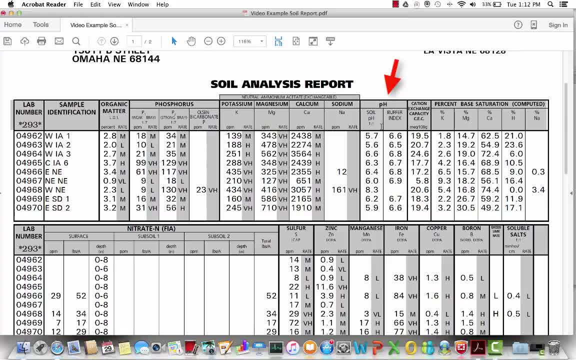 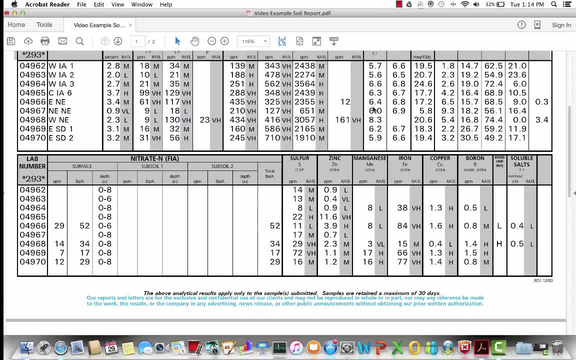 You know, as you deal with crops maybe like a lower pH environment. you'd certainly want to be there. I'm not an expert in the berries, but some of the berries like a lower pH environment somewhere. On the other hand, the buffer index is actually looking at your soil. 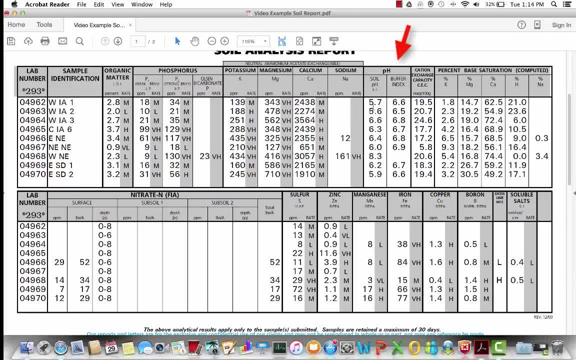 as we mix it with a known pH highly buffered solution, And then we look at the change in that solution's pH when we add your soil to it. So a heavier soil with more clay content will have a larger effect on this buffered solution than will a lighter soil with more sand in it. 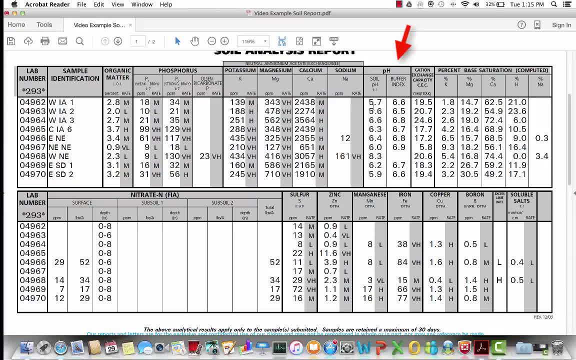 if the two soils had the same pH. So, starting with the soil pH here on the samples, we see we've got several here that probably could use some liming. As you look at the first couple, we've got pHs in that 5.6 and 5.7 area. 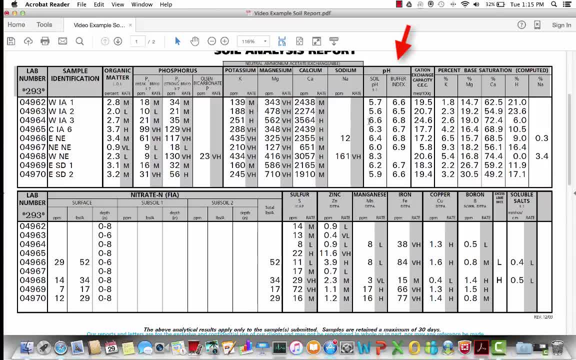 And like I said before on corn and soybeans, which is what we grow on this area, with these samples we'd probably like that to be more like around 6.5.. So we'd certainly make a lime recommendation Here. we've got a soil with a pH at 6.6 already. so not a lot of need for additional lime, but maybe you'd want to make a small application or maybe, say, a pell lime application, to try to keep the pH in that range that you're in already. We know as we add fertilizer, especially nitrogen fertilizers, 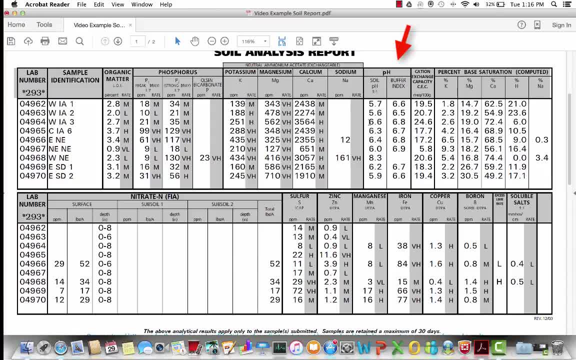 they add hydrogen to the soil And that additional hydrogen of course increases the acidity And that's what we're measuring. when we're measuring soil pH is that 6.6.. So we've got free hydrogen in the soil. that's a lot of times going to come from our fertilizer applications. 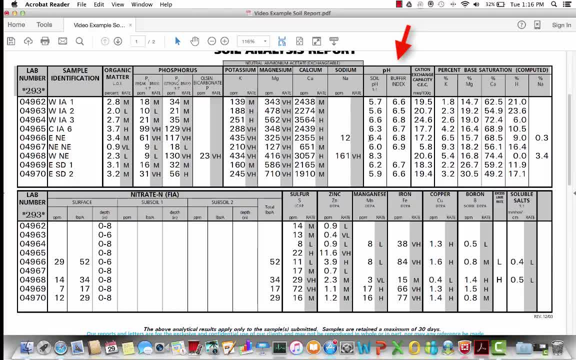 As we go down the rest of these samples, the central Iowa to 6.3, the eastern Nebraska to 6.4, kind of in that range that we'd like to be at. But again you might consider some small applications just to keep them there. 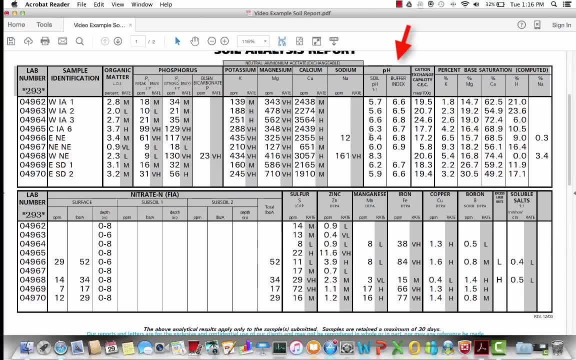 knowing that as you add fertilizer, especially nitrogen fertilizer, say for corn, you're going to be bringing that pH down and increasing the acidity with that additional hydrogen coming from the fertilizer applications. The one here, we're going to go down the rest of these samples. 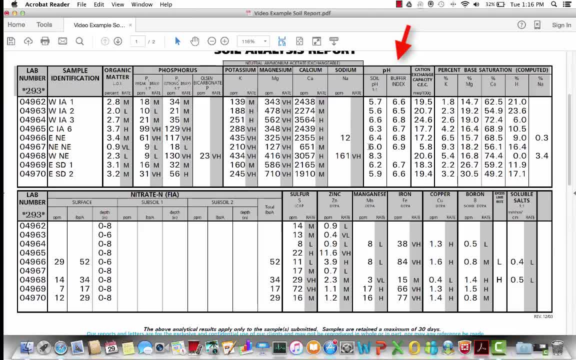 Northeast Nebraska, which again was that one with a very light CEC, is at 6.0. And maybe we would say that it's just a low edge of where we'd want to be. But we know that additional fertilizer application is probably more likely to move this pH down quicker. 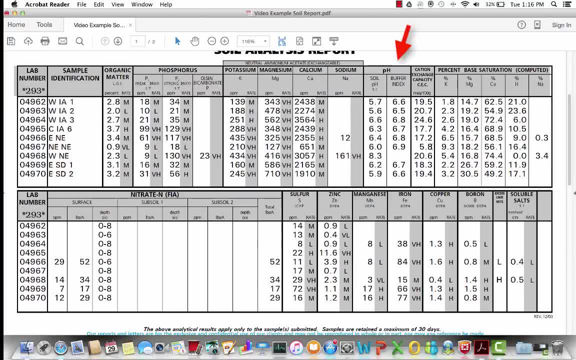 because it has less buffering capacity against those pH moves that would come from the cation exchange capacity and its overall- again- nutrient holding abilities. So adding that additional hydrogen with some additional fertilizer, it's probably going to bring this one down more rapidly than a lot of the soils around it. 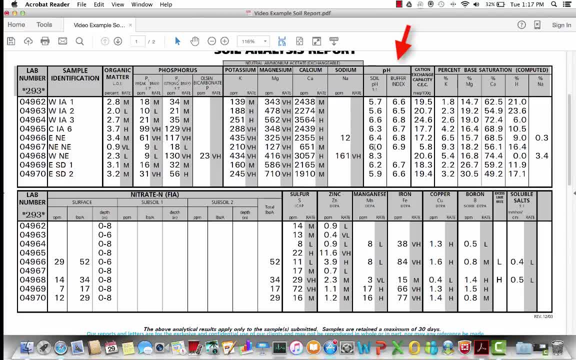 So we might want to jump in on that one and get that lime application made here in the soil. Of course we have a high pH soil with an 8.3 here. Higher pH soils can be difficult to grow some crops in. You run into some issues with nutrient tie-up a lot of times. especially with nutrients like phosphorus and some of the micronutrients, But they can also be very productive soils. You just want to understand that. You want to understand some of those issues that you can have in a high pH soil, and that's why we certainly make that measurement. 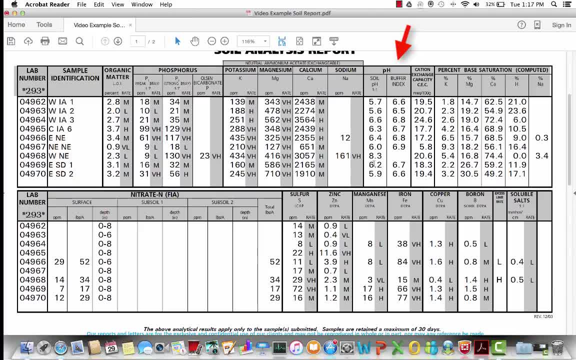 And then on the 6.2 pH here probably a pretty decent area to be in for, say, corn and soybeans, but getting toward the lower end of where you'd want to be Again, we'd like to be more like around 6.5,. 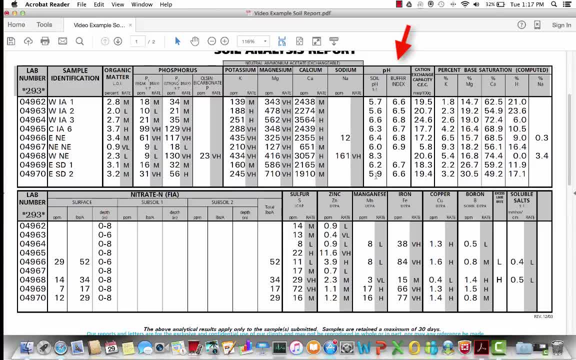 so we might consider some application there And here we're below 6.0 again. so with a pH of 5.9, lime probably should be applied to try to bring it up to somewhere around that 6.5 range. And again, some of this is going to depend. 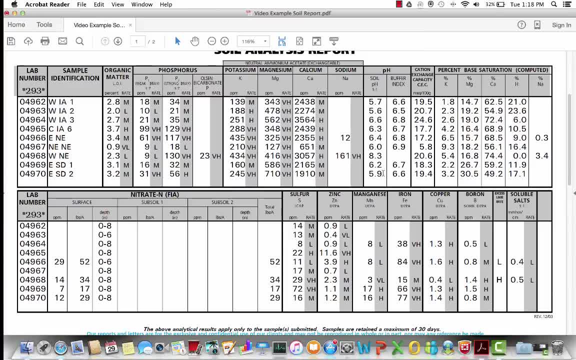 on your tillage. If you're doing no-till, you might want to take some separate samples that are shallower to look at that pH and that top of the soil environment where you might have changes greater than what you would see with an 8-inch sample. 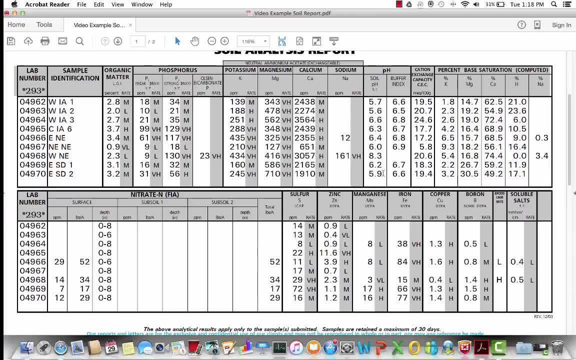 So that's something a lot of the growers that we work with will do- is they'll take a separate sample at 0 to 3, check pH on that and then also check the pH at, say, 0 to 6 or 0 to 8,. 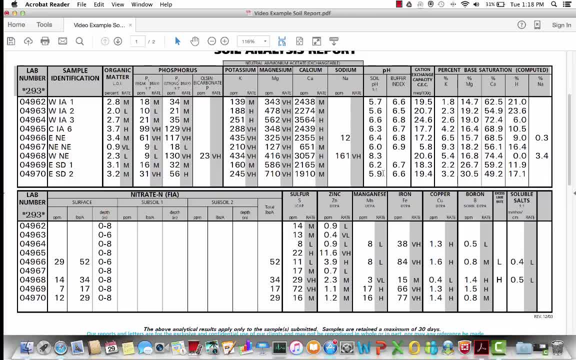 where they would normally make their lime recommendations. When we move over to the buffer index, you'll see here, with the high pH soil, we do not have a buffer index. That's because when pHs are above about a 6.8 or 6.9,. 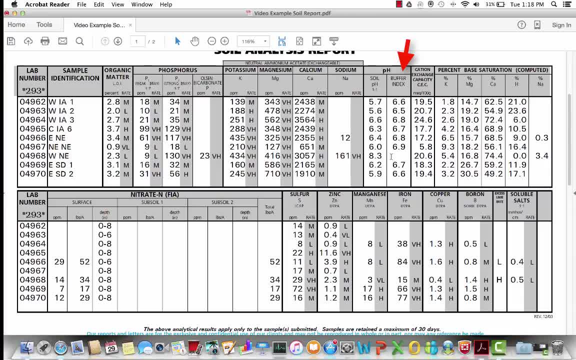 we do not run the buffer. We assume that you will not be liming that soil to try to increase the soil pH, so no buffers run. And that's the case of this soil with the 8.3 pH. As we look across these other soils, we've got buffer indexes ranging from a low of 6.5 to a high of 6.9.. Now here's an interesting thing that kind of makes the case that I was talking to you earlier about how the buffer index can differ a lot based off the pH. 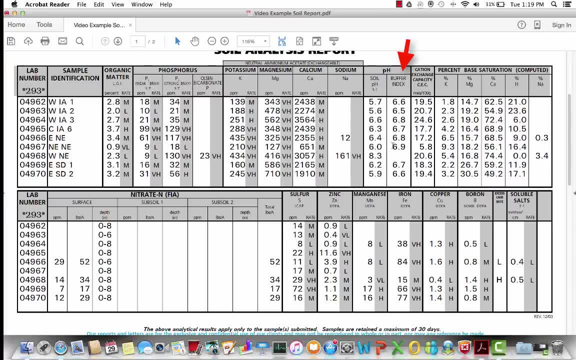 of the soil, but also based off of that cation exchange capacity or the buffering capacity of that soil. We see a soil here with a pH of 6.3, a little lower, and it's got a buffer index of 6.7.. 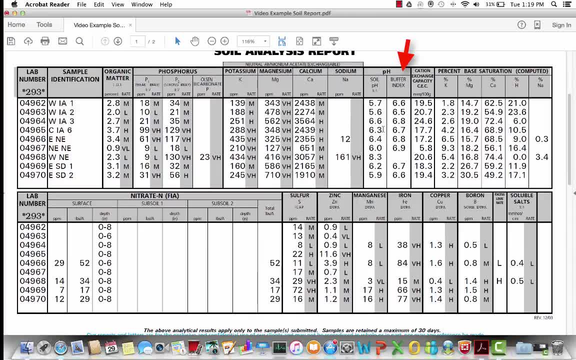 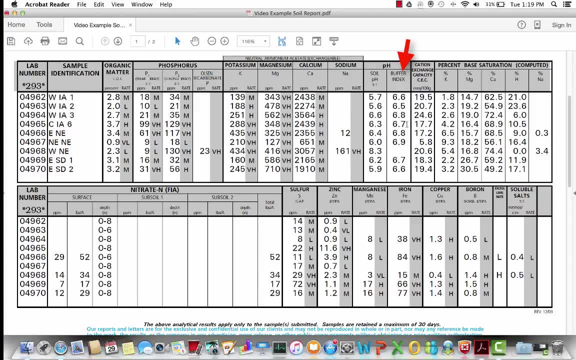 But here we see a soil with a pH of 6.0, which is, you know, significantly lower than the 6.3 and 6.4 soils above it, but the buffer index is actually higher than the two soils above it. 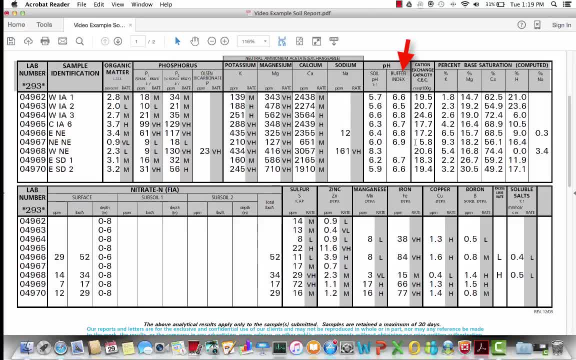 And again, that has to do with that texture of the soil and its cation exchange capacity. The hydrogen that we're measuring here, with this pH of 6.0 overall in that soil is actually less than it is in the other two, because, again, there's just less exchange sites. So even though the active hydrogen is bringing the pH down, the pH is going to be lower. The total amount of hydrogen or that reserve acidity that we need to correct with our lime recommendation is actually less than the two soils above it. 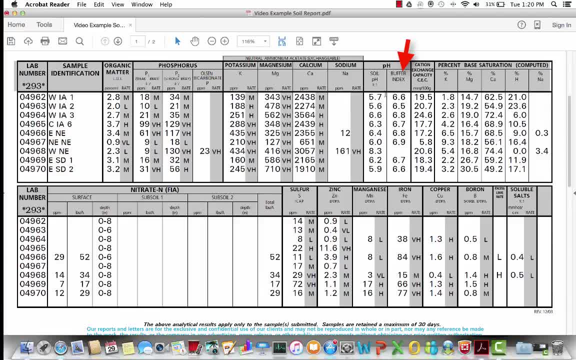 And that's why we run the buffer index and we do not recommend that people make lime recommendations solely off the soil pH, but instead use the soil pH as maybe a trigger to make the decision that, yes, I need to lime, but let the buffer pH be related to your actual recommendation. 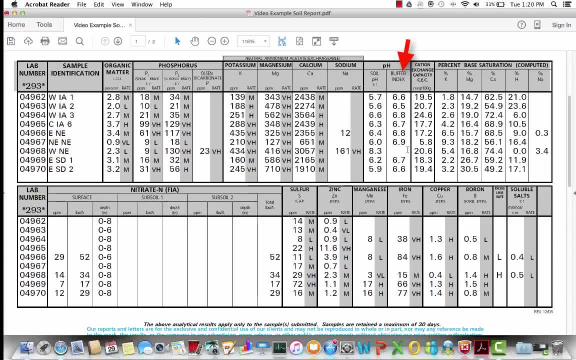 And if you go to, say, Iowa State, Iowa State's Guide to Lime Recommendations and Fertilizer Recommendations, they would give you recommendations based off these buffer indexes for actual lime application. Or, of course, you could ask the lab for our recommendations. So again, soil pH is actually the pH of your soil, Say, for a corn-soybean rotation. we'd certainly like that to be around that 6.5, just say 7.2. Once you start running the low sixes, or certainly below six, 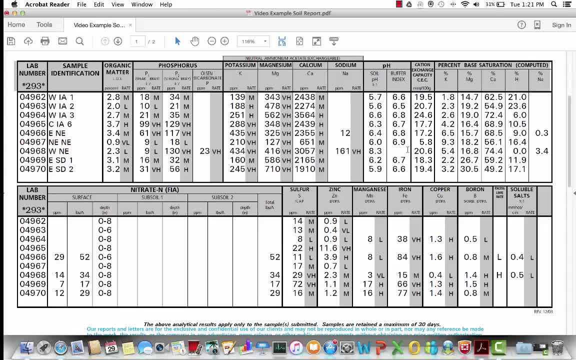 you really should be thinking about making some lime application. But when you go to make that lime application, instead of using just the soil pH, you would want to use the buffer index, which will take into consideration both the free hydrogen that's in that soil.